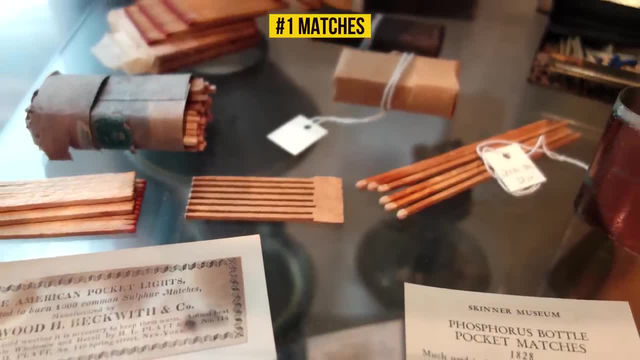 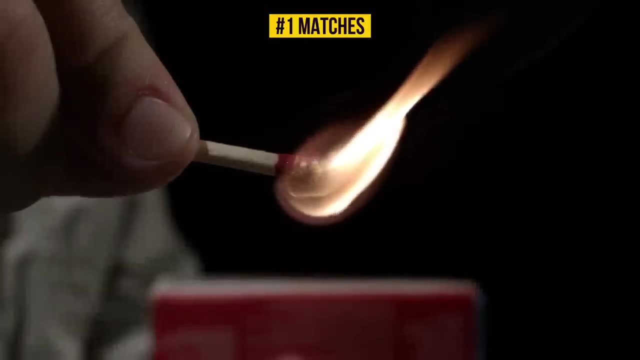 He started making and selling these cardboard matches, which he later replaced with 3-inch wooden sticks accompanied by a piece of sandpaper to light them. Walker humbly decided not to patent his invention because he believed it would be easier for him to benefit humanity. 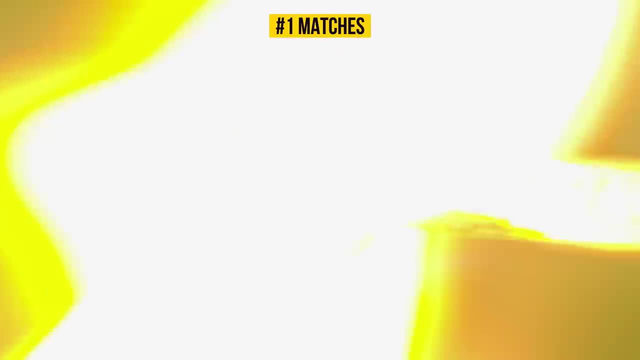 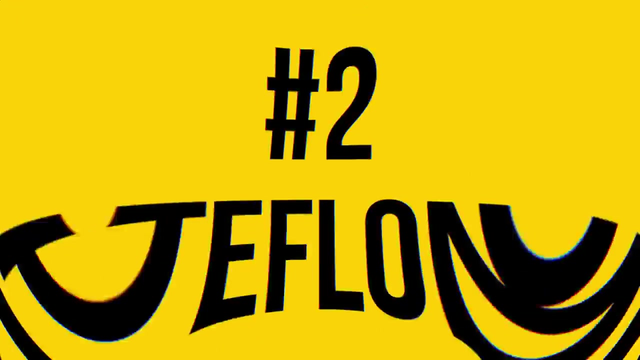 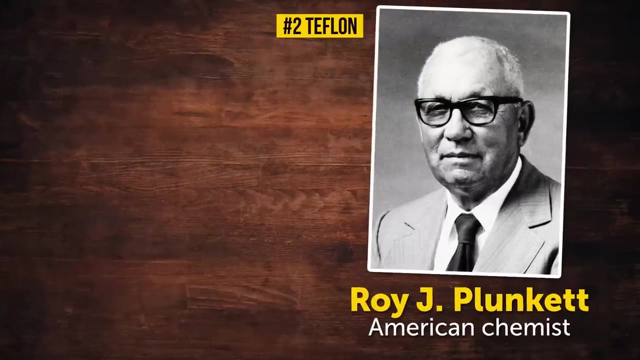 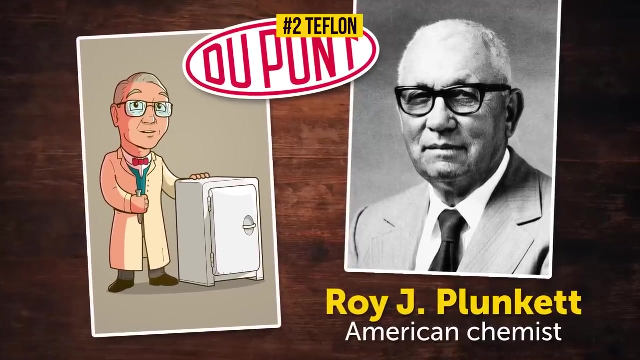 so he decided to make a commodity this way. Matches soon became popular all over the world and are still a useful commodity today. Teflon American scientist Roy J Plunkett was doing research for the company DuPont with a goal of finding a way to make their fridges safer by replacing the hazardous refrigerant Freon with something else. 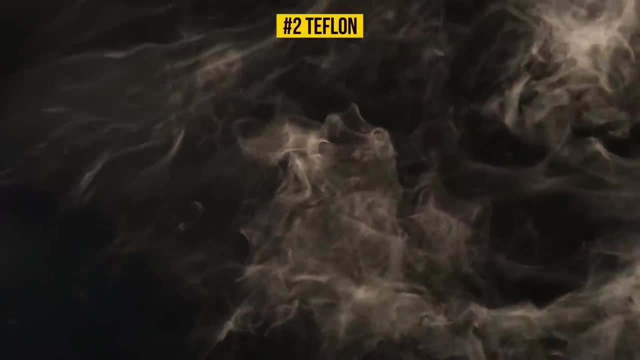 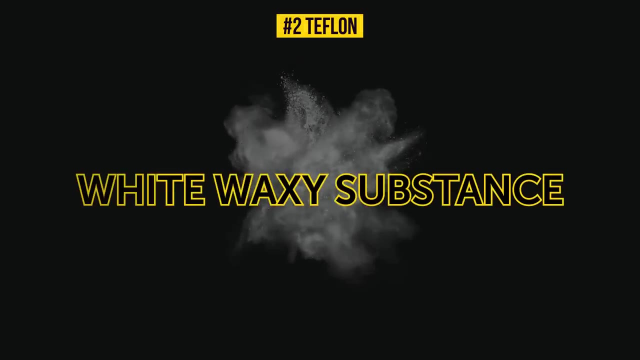 He must have thought it was another failed experiment when he found that the gas mixture he had created just vanished overnight, and all that was left of it in the container was some white waxy substance. That strange substance proved to have some useful qualities. 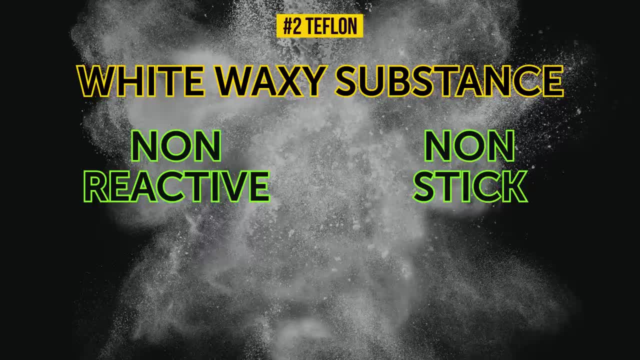 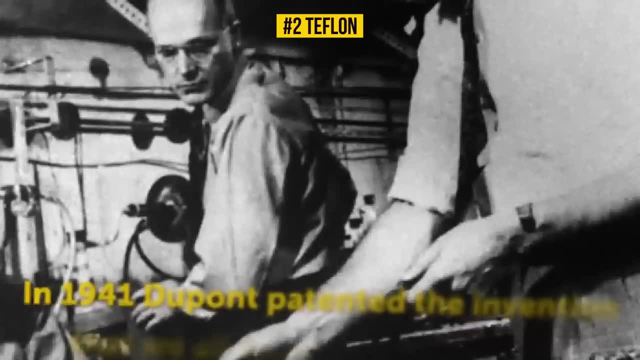 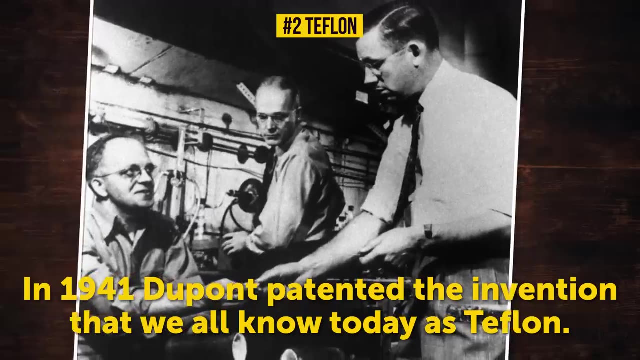 It was non-reactive, non-stick and resistant to extreme temperatures from minus 100 degrees to 500 degrees Fahrenheit. In 1941, DuPont patented the invention that we all know today as Teflon. The Teflon was a very important tool in the world of cooking. 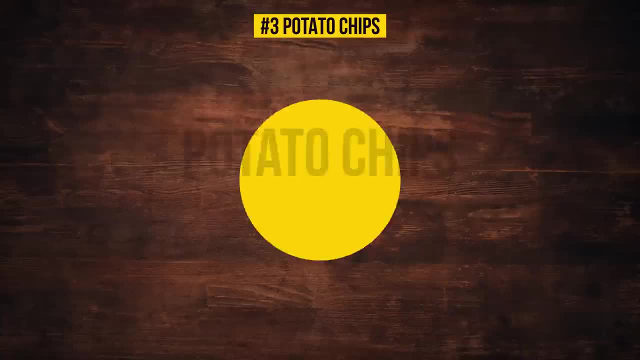 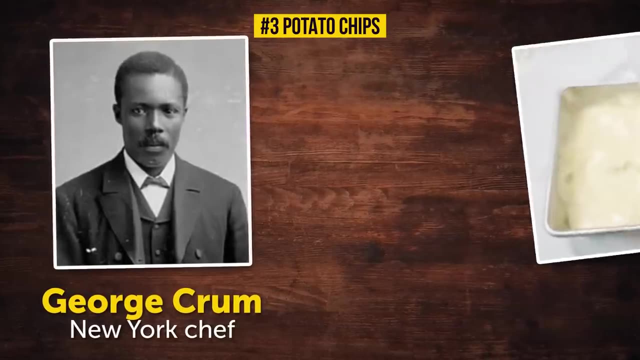 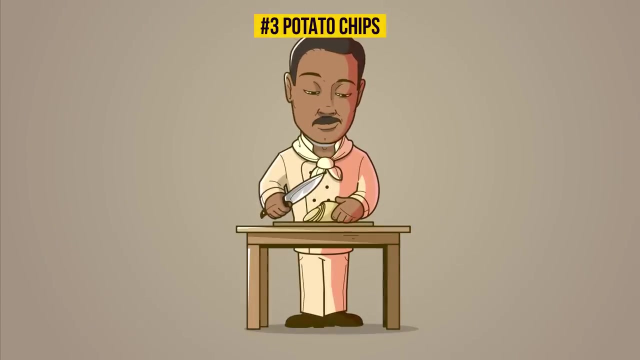 Potato chips. New York chef George Crumb. Great name for a chef. huh Actually it'd be better for a baker. Anyway, chef Crumb got a lot of customer complaints that his fries weren't crispy enough. Crumb a bit annoyed. 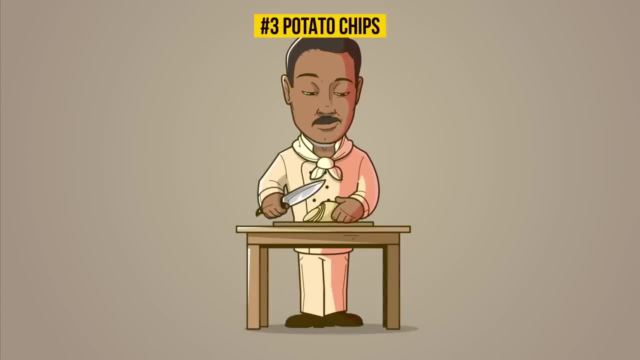 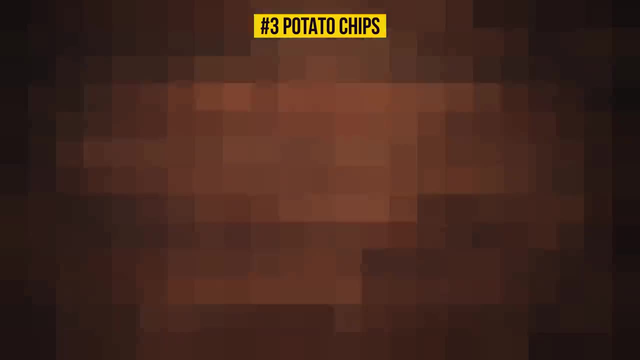 decided to slice the potatoes as thin as he possibly could, deep fry them in boiling oil and slather them in salt. That ought to show him, he pointed. he probably thought, But to his surprise people went crazy for the new recipe. 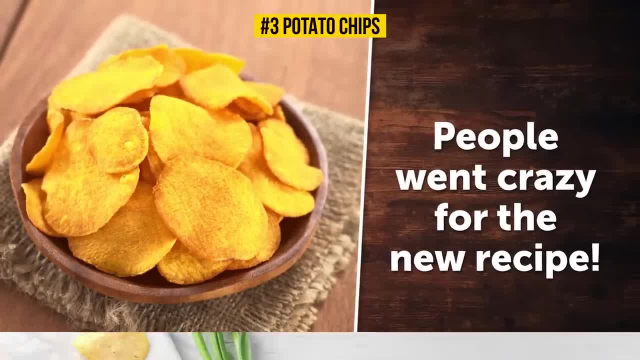 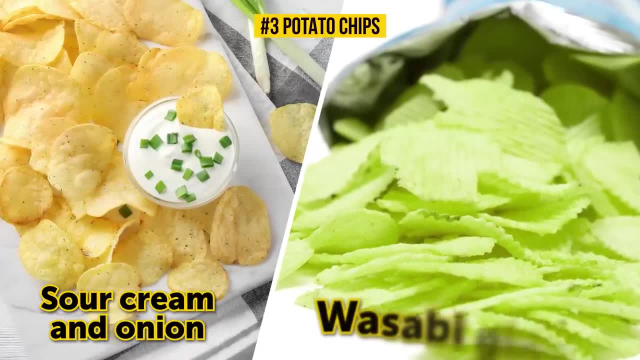 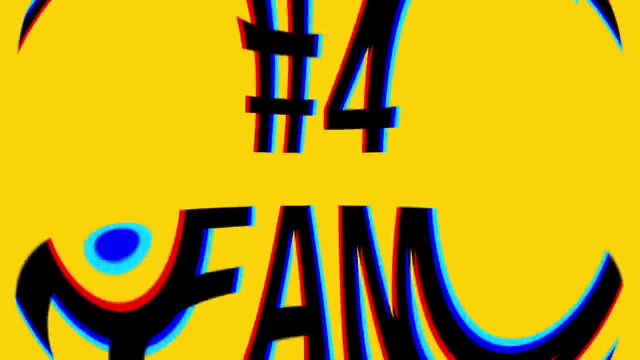 Potato chips have changed a lot since 1853.. Today they come in over 200 different flavors, from the classic sour cream and onion to some pretty bizarre ones like wasabi, ginger- Ooh, that sounds good. Ice cream cones. Ice cream itself is nothing new. The Chinese ate something very similar to it as early as 200 BC. Ice cream cones, however, were the product of a happy accident at the 1904 World's Fair in St Louis. The ice cream booth had been so rushed with customers. 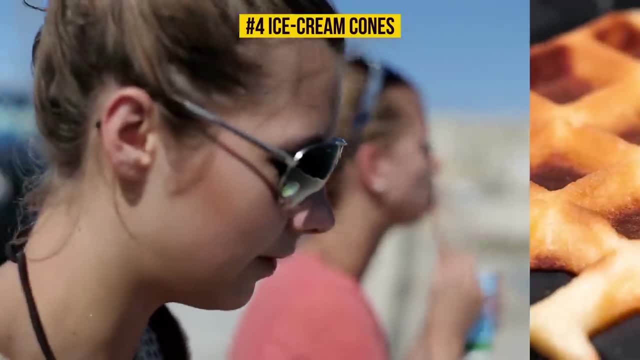 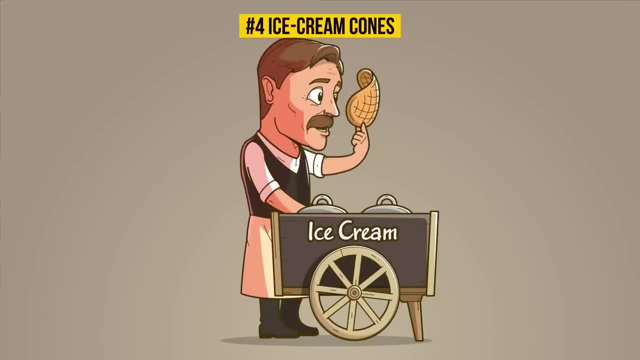 that it ran out of bowls. Things weren't so busy in the next booth over where Ernest Hamway was selling Persian waffles. In a kind gesture, Hamway started rolling his waffles up into cones and offered them to his neighbor to use instead of bowls. 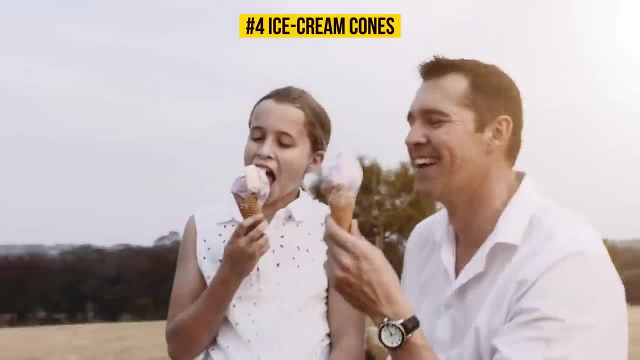 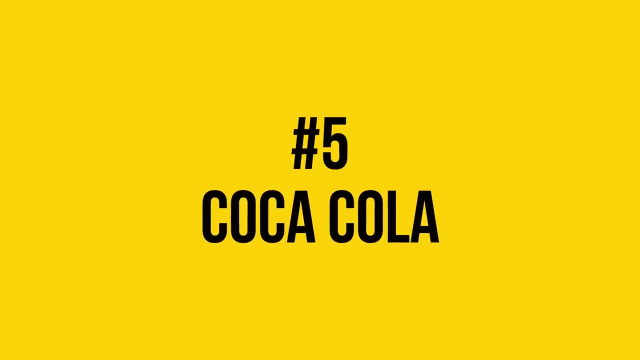 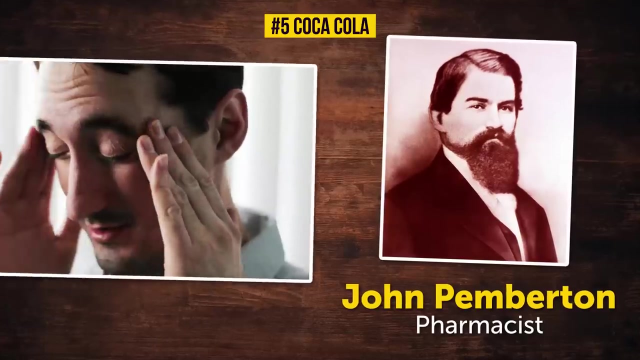 Customers fell in love with the final product, and that's how the ice cream cone was born- Coca-Cola. John Pemberton wasn't a businessman. He was just a pharmacist trying to find a way to get rid of headaches. So he came up with a simple recipe. 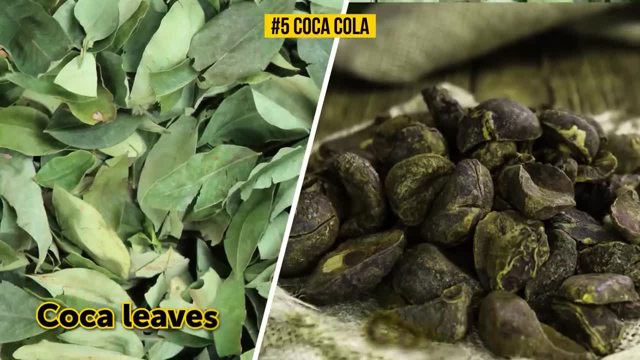 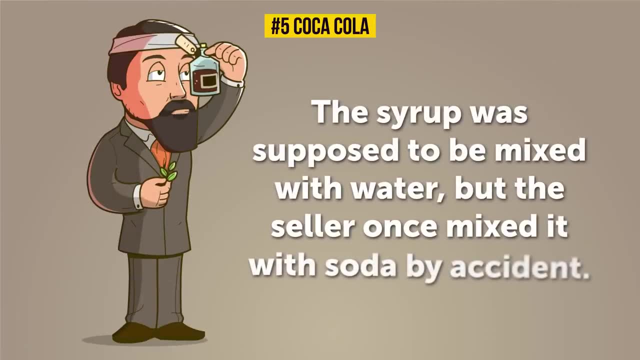 consisting of two ingredients: coca leaves and cola nuts combined into a syrup. It went on the market in 1886.. The syrup was supposed to be mixed with water, but the seller once mixed it with soda by accident. This is how the delicious and refreshing drink. 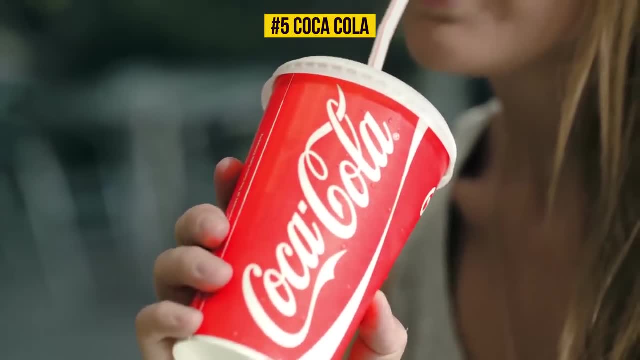 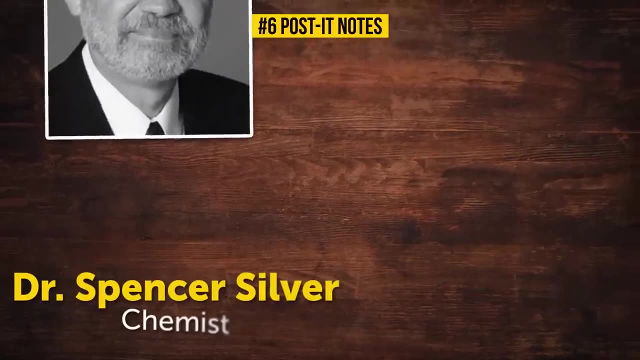 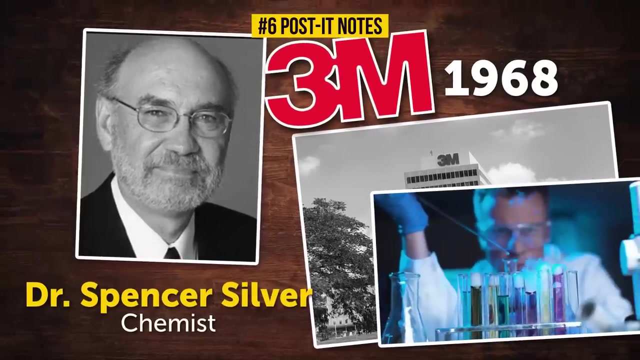 we all love today was created: Post-it notes. Dr Spencer Silver was working as a chemist for 3M Company back in 1968. He was trying to create a super-strong adhesive, but when he got it he got instead was quite the opposite. 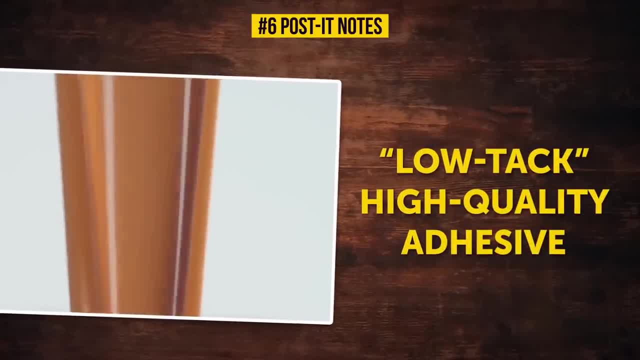 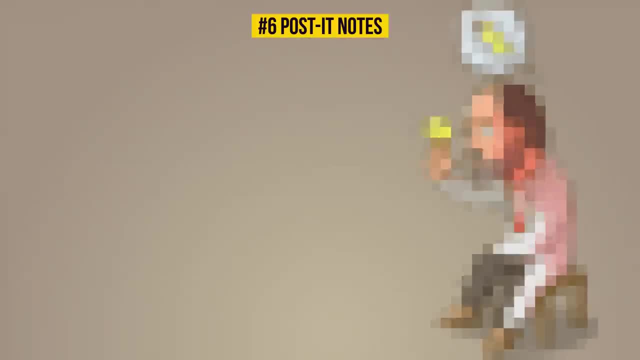 A low-tack yet high-quality adhesive: only strong enough to hold up a piece of paper, but durable enough to be relocated multiple times without losing its stick. It wasn't until 1974 when the use for his invention was found. His colleague needed something. 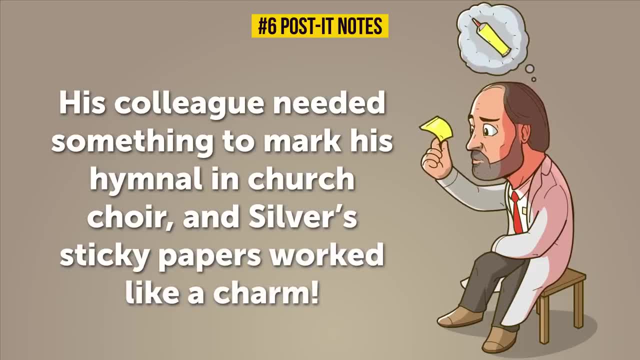 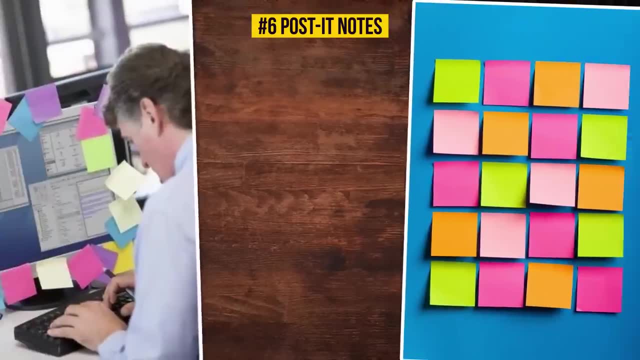 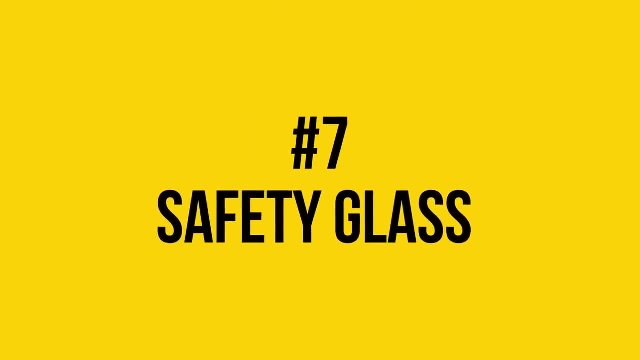 to mark his hymnal in church choir, and Silver's sticky papers worked like a charm. The name Post-it Notes was later dubbed and they became a must-have in homes, schools and offices around the world. Safety Glass. French chemist Edouard Benedictus. 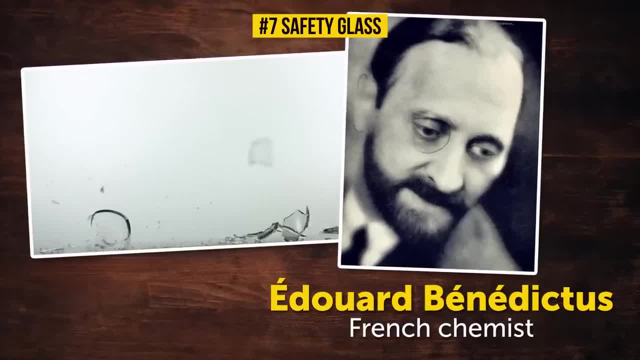 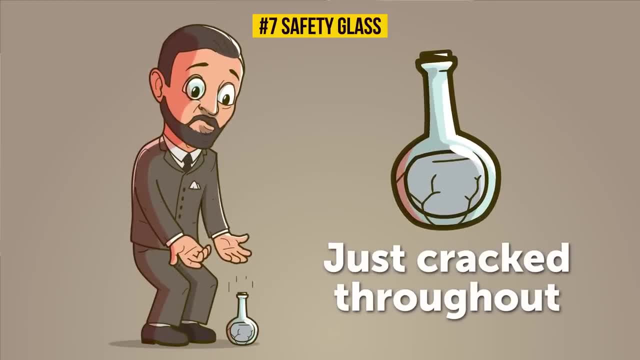 once accidentally knocked a beaker off his desk. To his surprise it didn't shatter into pieces, but just cracked throughout. He couldn't figure out why until he noticed that the beaker had had a thin film of liquid plastic in it, left over from a previous experiment. 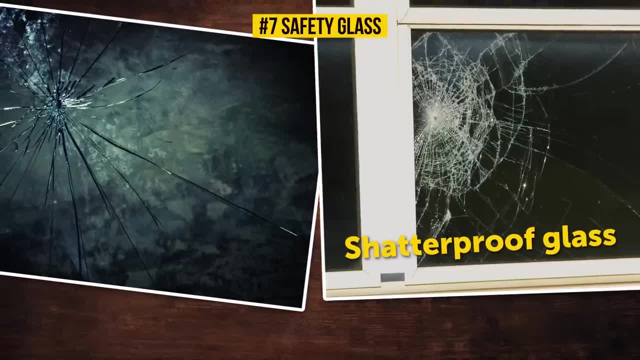 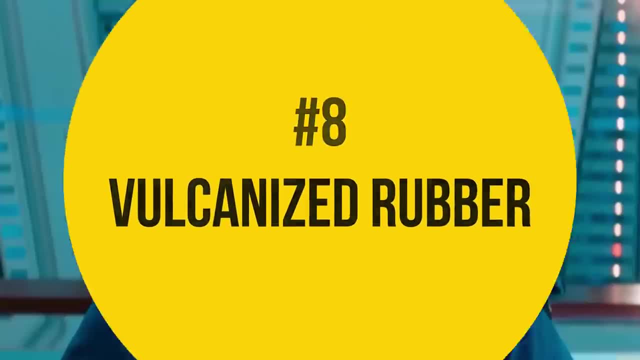 And this is why he called it a beaker. And this is why he called it a beaker. This is how shatterproof glass was invented. Vulcanized rubber: No, it was not invented by Mr Spock, A young scientist named Charles Goodyear. 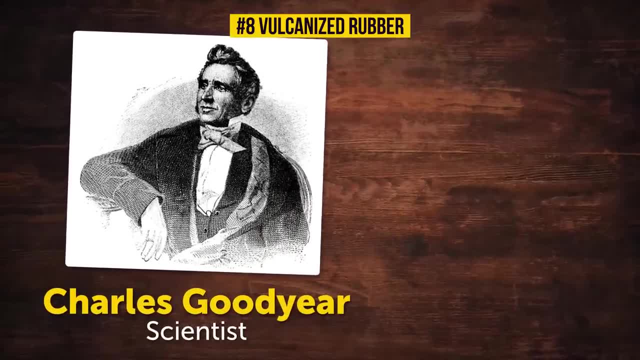 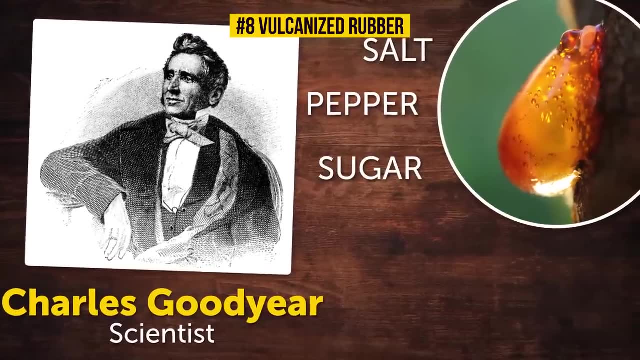 was trying to improve the quality of rubber, which wasn't so durable. in the 19th century, Goodyear was experimenting and mixing raw resin with salt, pepper, sugar, sand, castor oil and even soup in an attempt to find the perfect combination. 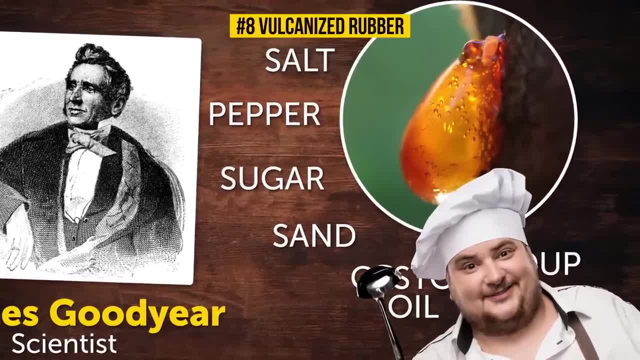 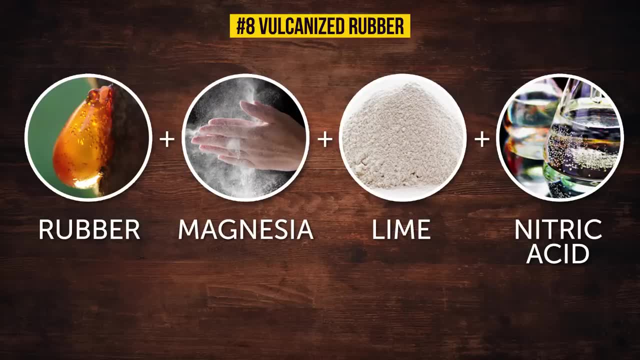 Sounds like he was really trying to invent lunch. Anyway, one day he decided to see what would happen if he mixed the rubber with magnesia, lime and nitric acid. Again failure. But once the rubber was mixed with sulfur and accidentally dropped on a hot surface. 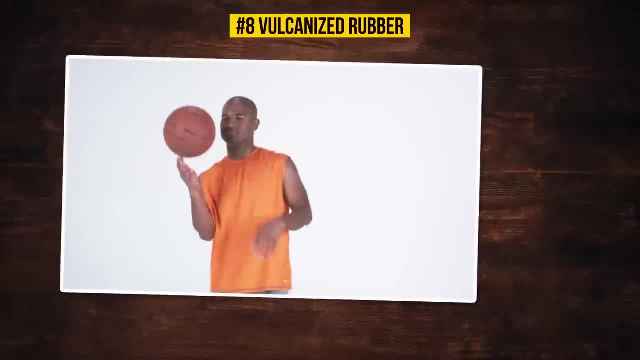 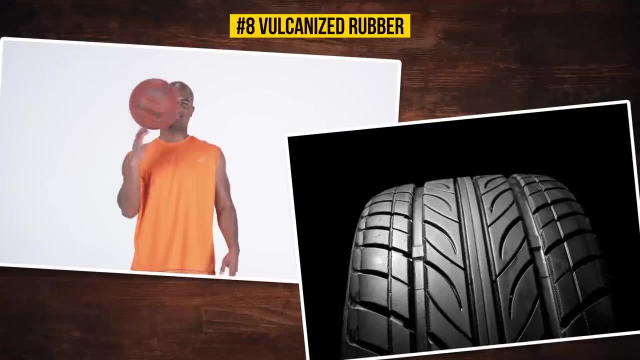 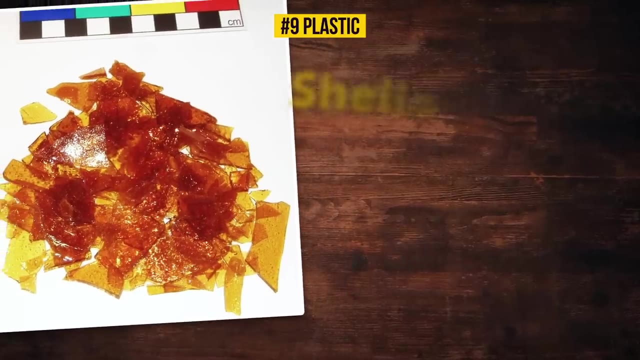 it worked. The scientist invented vulcanized rubber. that's now used to produce just about everything from basketballs to car tires- Plastic. Before we had plastic, there was shellac. It was used in the beginning of the 20th century. 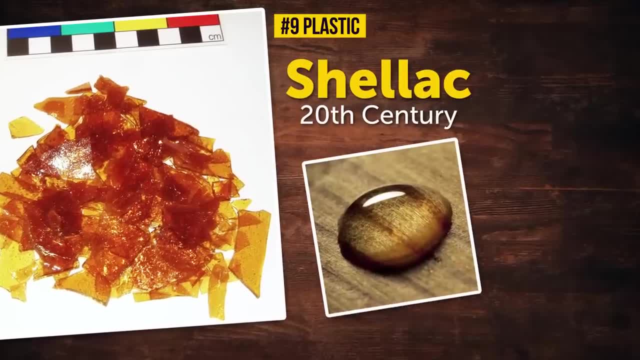 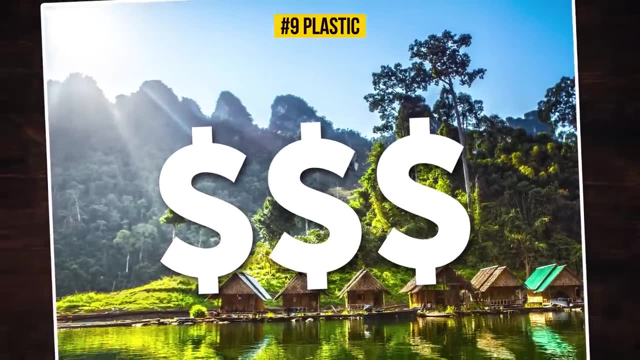 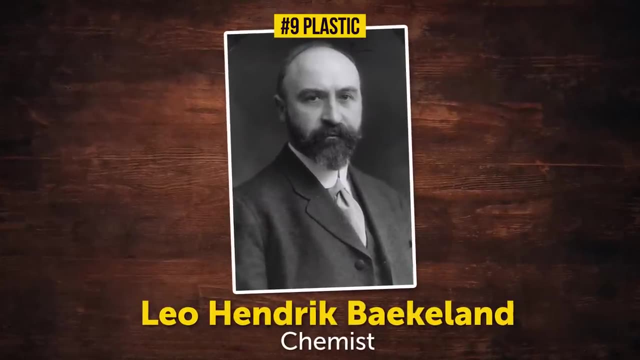 for all kinds of purposes, from wood varnishing to making records and even dentures. The problem was its price. It was super expensive to import beetles from Southeast Asia for its production, So chemist Leo Hendrik Bekeland tried to find a cheap way to make it. 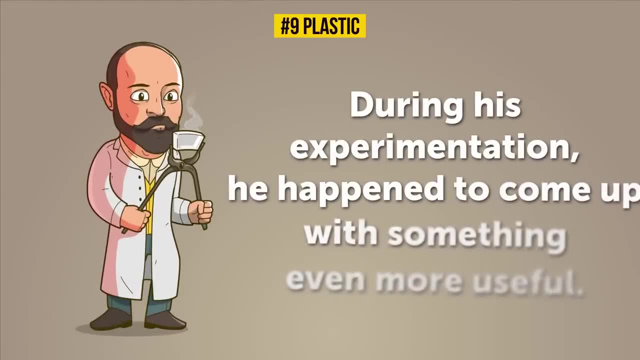 But he couldn't. He tried to find a cheap way to make it. He tried to find a cheap way to make it. He tried to find a cheaper alternative for shellac. During his experimentation, he happened to come up with something even more useful. 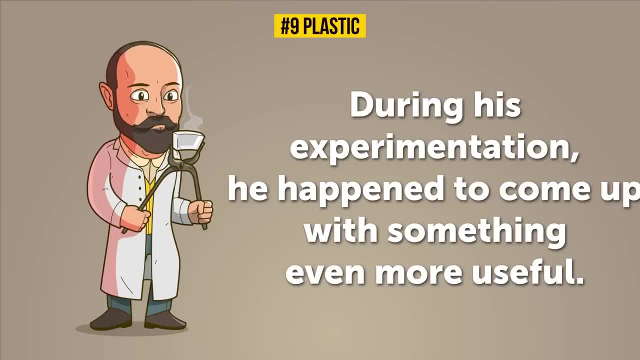 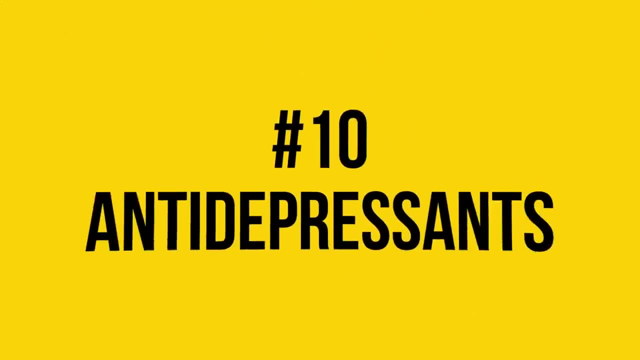 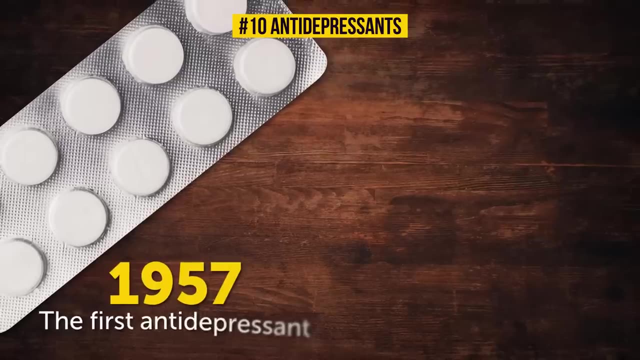 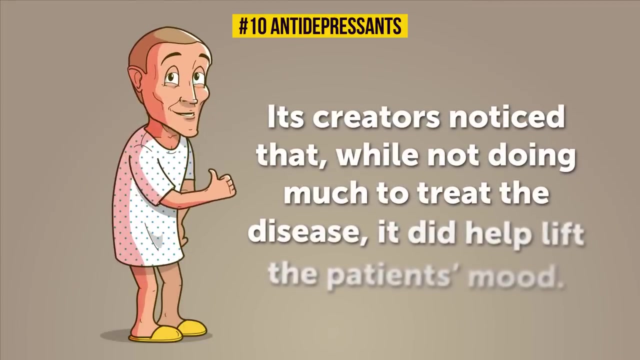 The new mixture was a moldable material able to resist extremely high temperatures. We all know it as plastic Antidepressants. The first antidepressant was discovered in 1957 and was supposed to be a cure for tuberculosis. Its creators noticed that, while not doing much, 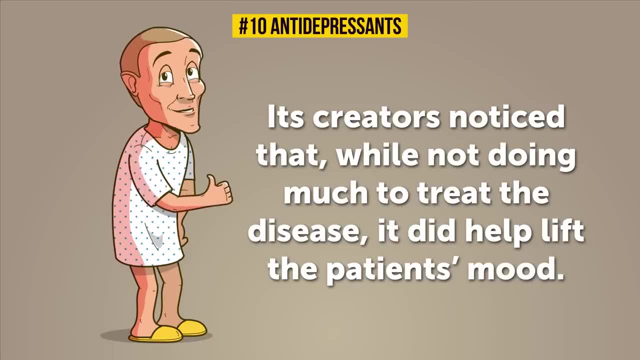 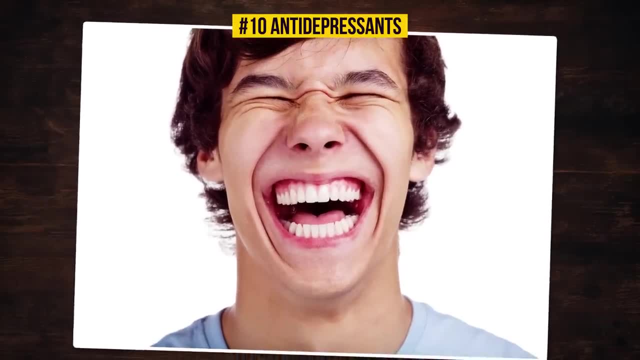 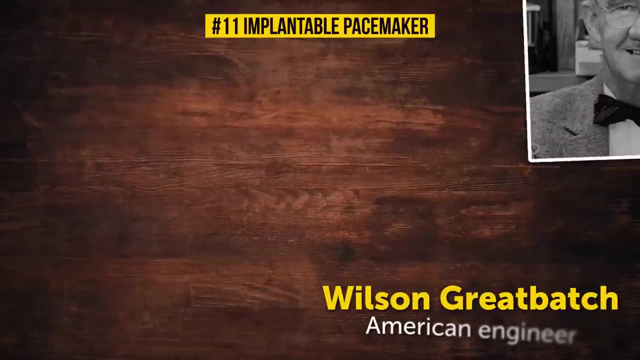 to fix the disease. it did help lift the patient's mood And we still use this medicine to treat the symptoms of depression today. Implantable pacemaker Wilson Greatbatch was trying to create a device that would simply record the human heartbeat. 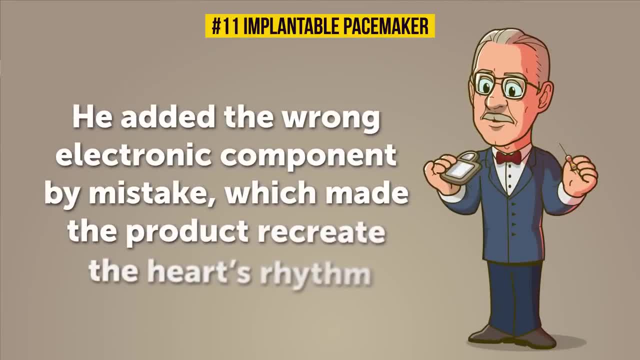 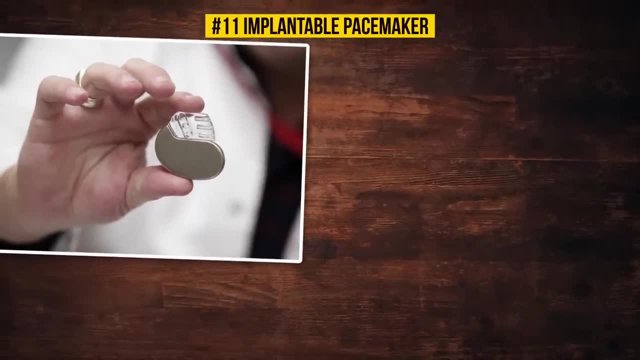 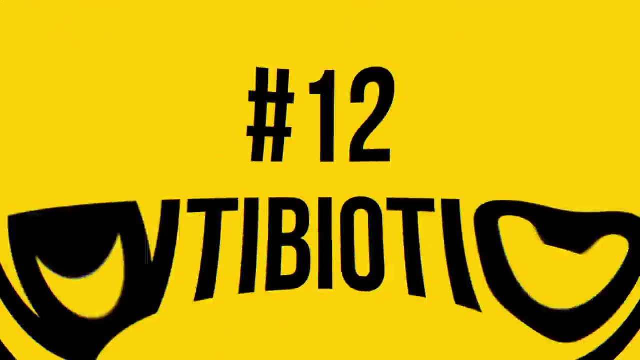 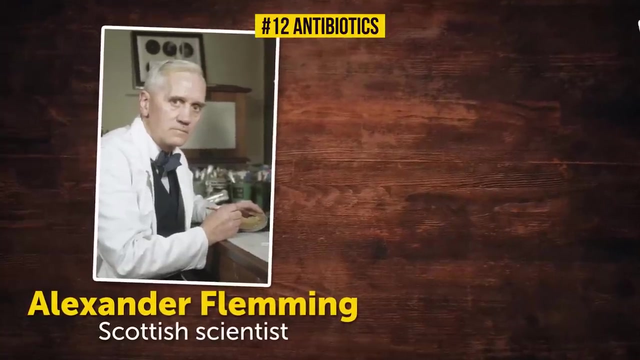 He added the wrong electronic component by mistake, which made the product recreate the heartbeat. This pacemaker was successfully implanted in the first human in 1960 and has been saving lives ever since. Antibiotics. Scottish scientist Alexander Fleming's laboratory was always a mess. 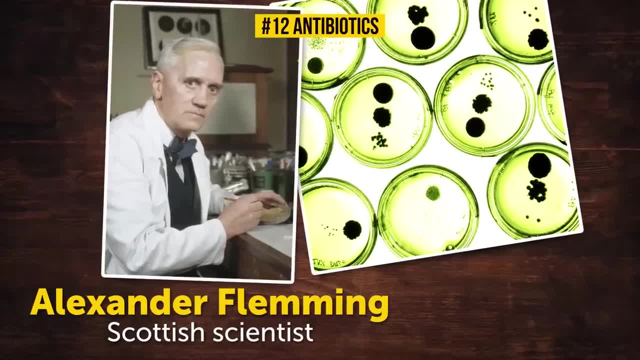 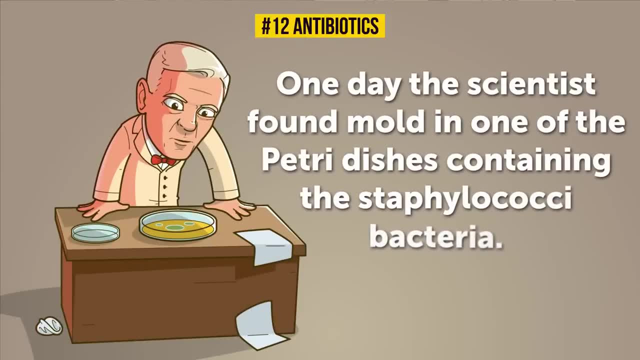 Beakers and papers all over the floor, a desk full of petri dishes with different kinds of bacteria. One day the scientist found mold in one of the bacteria's cells. The mold had formed a sterile shield around itself, killing the bacteria in the dish. 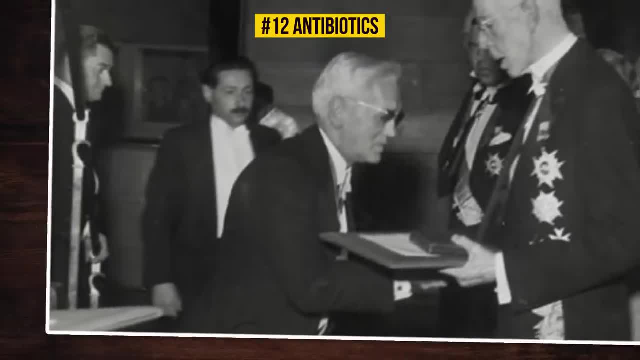 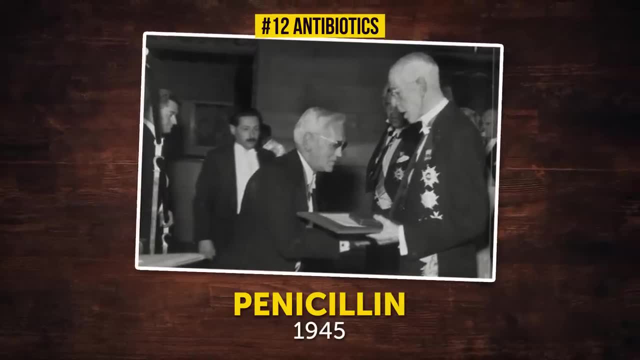 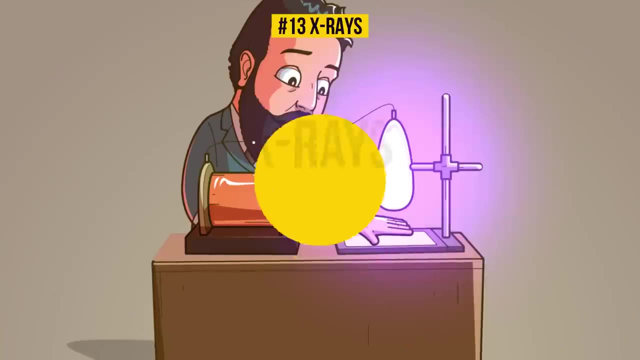 Fleming, intrigued, decided to further study the properties of this fungus. He received a Nobel Prize for the discovery of penicillin in 1945.. X-rays When Wilhelm Rentschen unintentionally put his hand in front of an electron beam tube. 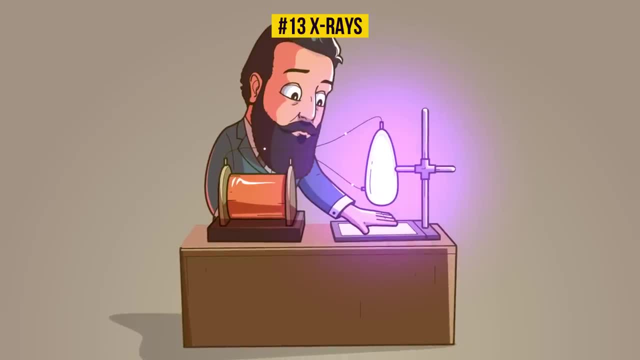 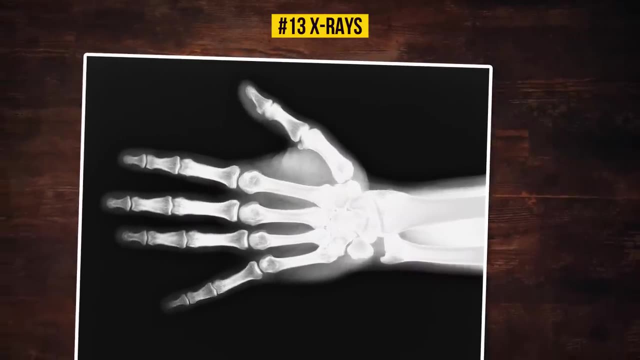 back in 1895, it fell off? No, not really, But he immediately saw an image of his hand on a photographic plate. He noticed that the radiation passed through solid objects and body parts, leaving a shadow The denser the object was. 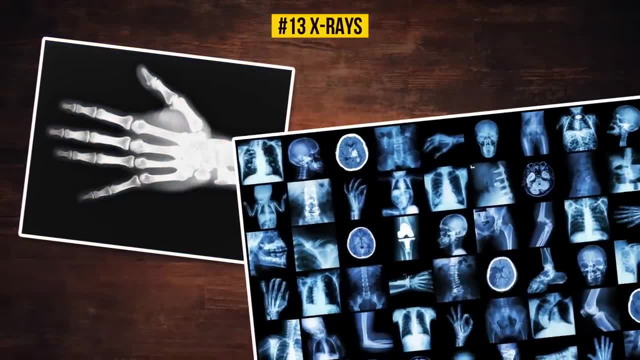 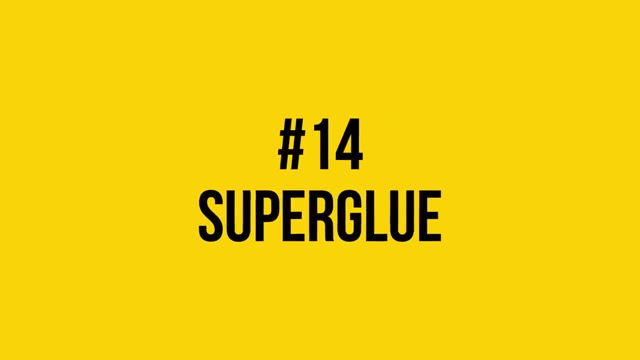 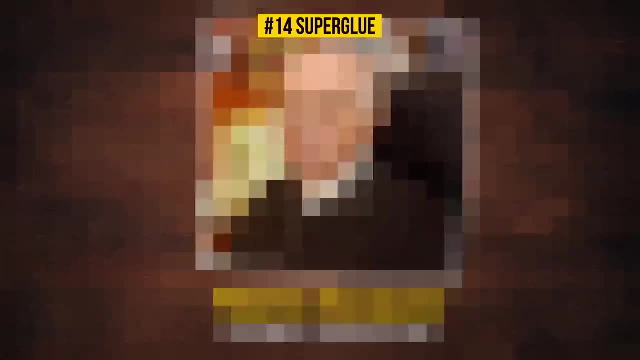 the more massive the shadow, And now we have X-ray imaging Superglue. In 1942, Kodak researcher Harry Coover was working on a transparent plastic for gun sights when he accidentally created an extremely adhesive substance that stuck to just about anything. 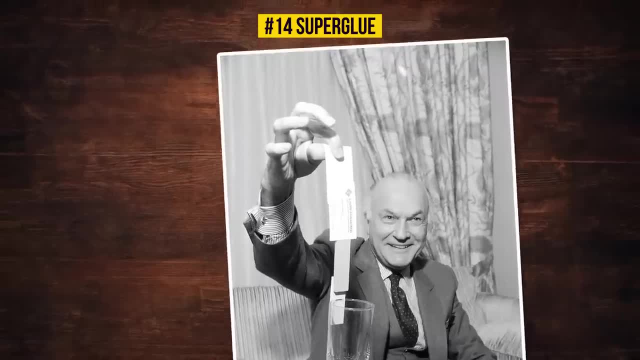 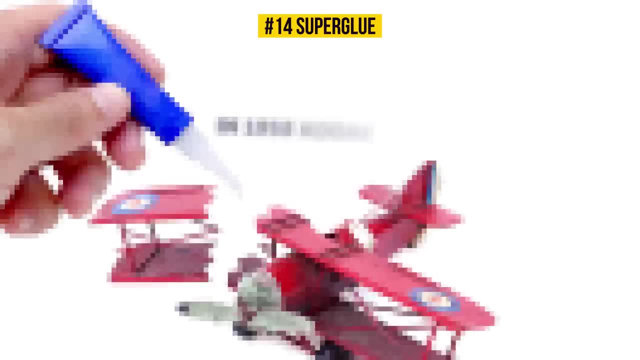 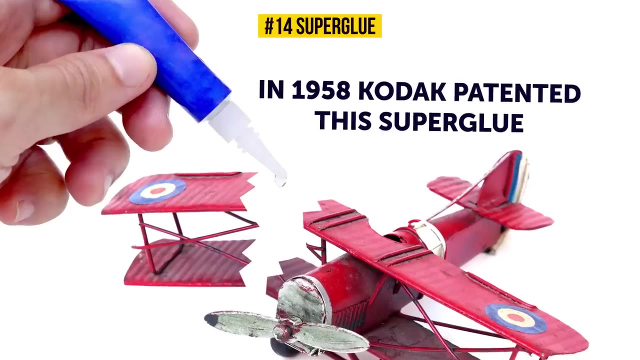 While working on another research project. sometime later, the adhesive again proved too sticky, Seeing this as both a unique and useful discovery. in 1958, Kodak patented this superglue. we all have a love-hate relationship with today, But it's not the end of the story. 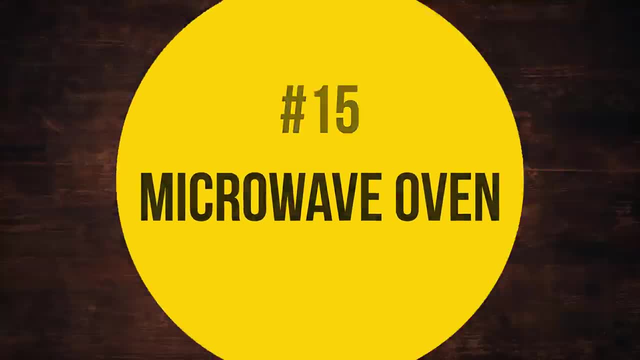 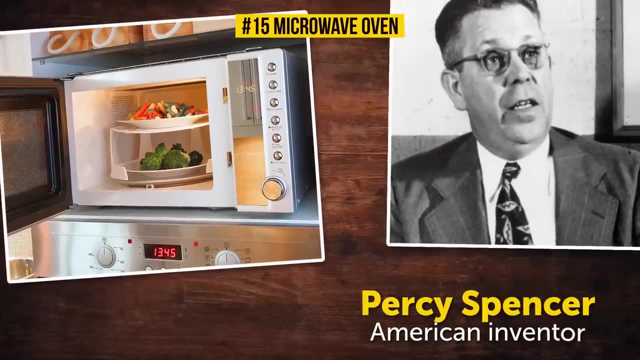 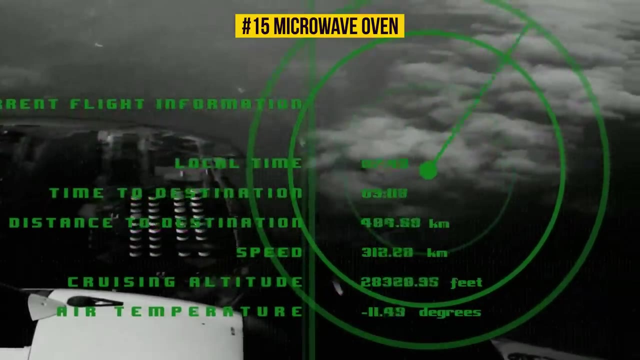 Microwave oven The next time you're heating up a meal or some popcorn in a matter of seconds, don't forget to thank Percy Spencer Back in his day. microwaves- not the kitchen appliance, but the waves themselves- were used in radar.